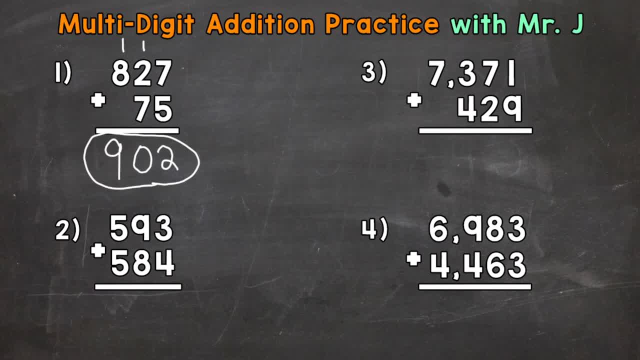 Let's start with the ones. So we have three plus four. That gives us a seven in the ones place. Now for the tens. we have nine plus eight, That gives us 17. So put the seven in the tens and regroup. 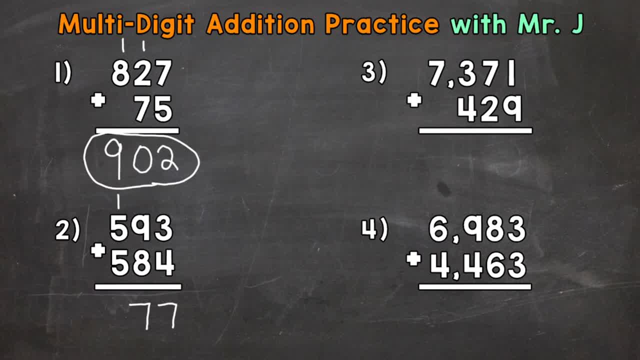 the one over to the hundreds. Now we have one plus five plus five in the hundreds, So one plus five is six, plus five is eleven, So one in the hundreds place and then regroup the other one over in the thousands place. Now 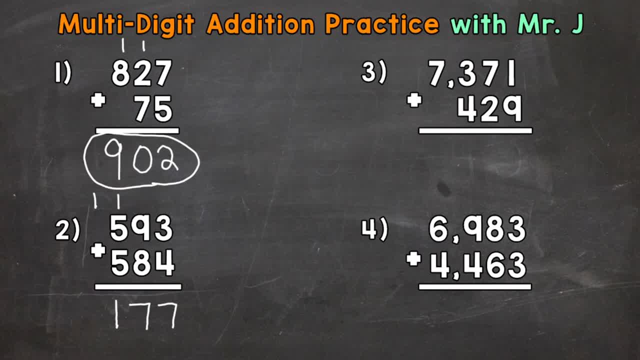 that one is the only thing in the thousands place. So we can bring it straight down: put a comma in our answer and our final answer is 1177.. Let's move on to number three, where we have 7371 plus 429.. 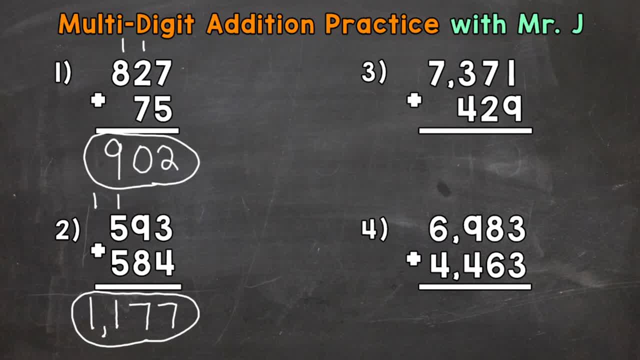 Start with the ones. So one plus nine gives us ten. Put a zero in the ones place And regroup the 1.. Now in the tens place we have 1 plus 7 plus 2. So 1 plus 7 is 8, plus 2 is 10.. So put: 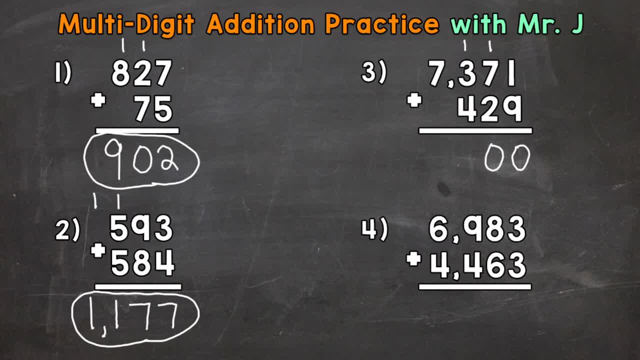 our zero in the tens place and regroup our 1. And now we add the hundreds So we have one plus three, So we could regroup one. And now we add the hundreds So we have one plus three plus four. 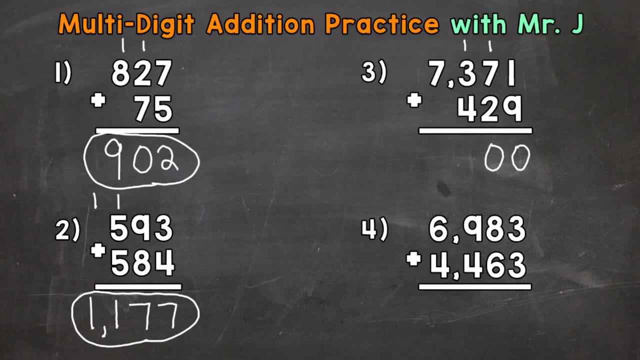 four. One plus three is four Plus four gives us a total of eight in the hundreds place. And then, lastly, the thousands place. we can bring that seven straight down, because we don't have anything else in the thousands. So basically, we're doing seven plus zero and we can just bring that. 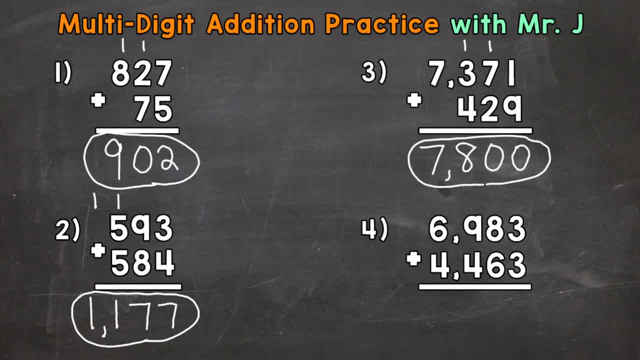 straight down for a final answer of 7,800.. Lastly, number four: 6,983 plus 4,463.. Add the ones: Three plus three gives us six. Now for the tens. eight plus six gives us 14.. So put our four in.